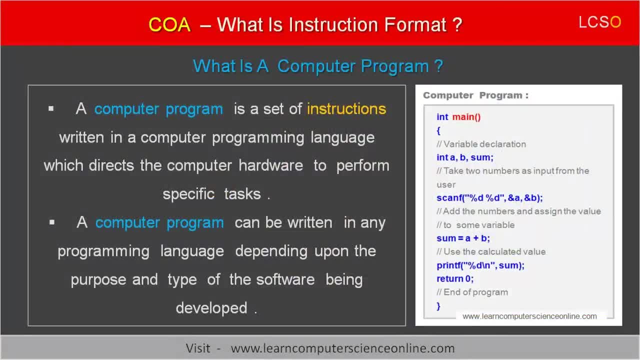 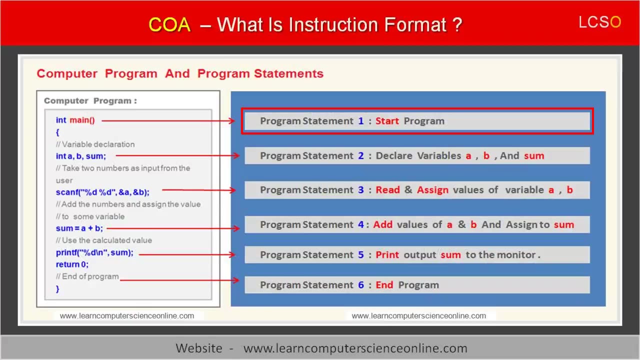 Every task performed by the computer needs a program. In other words, the computer is driven by the program instructions. A computer program consists of set of instructions. The program instructions direct the computer to perform the specific task. Each program statement performs a part of the intended operation. 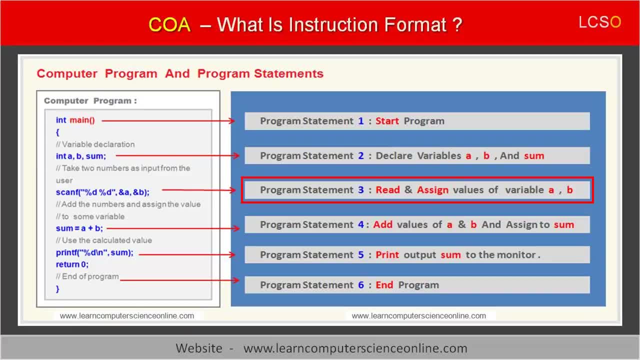 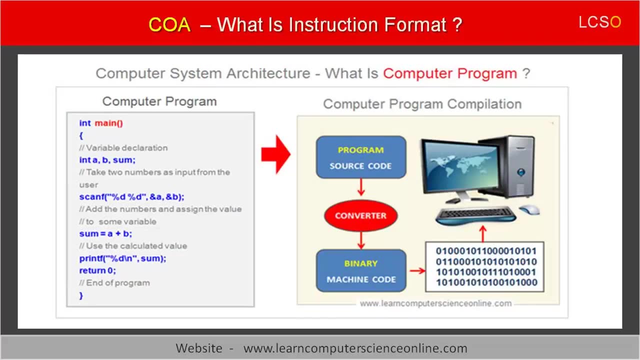 Each statement in the program is called as program instruction. However, the central processing unit, CPU of the computer cannot directly execute the program written in any high level language, such as Python, C++ and Java. The processor can execute only machine instructions in binary. 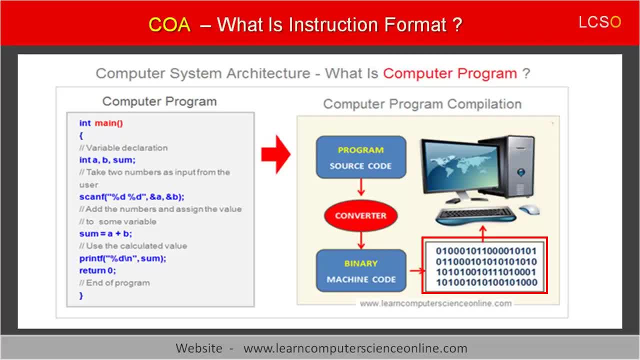 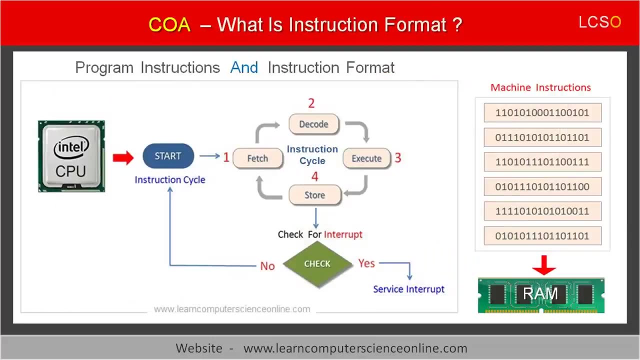 The binary code consists of only two digits, that is, zero and one, And therefore all computer programs are first compiled to binary format. The compiler translates the high level program statements into it's equivalent machine instructions in binary format. In computer architecture the instruction is defined as a machine instruction in binary that can be directly executed by the processor. 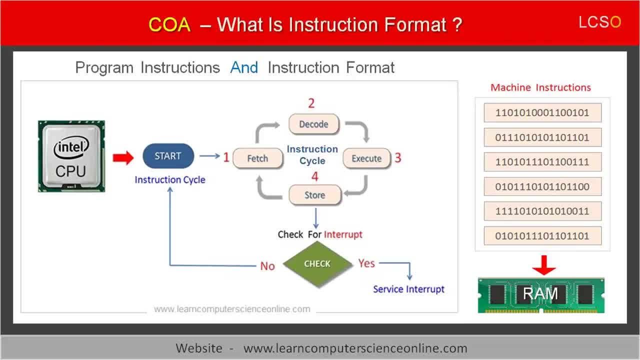 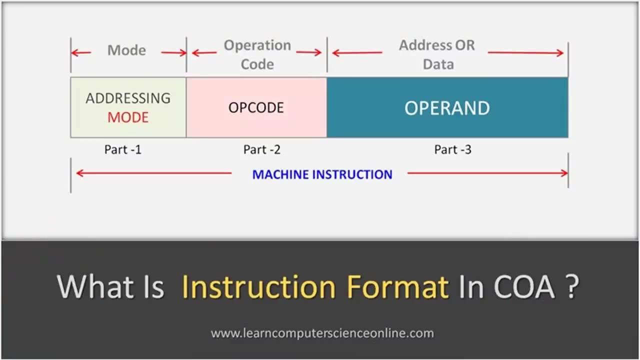 After the program compilation: each program instruction in binary format is called as machine instruction. instructions can be directly decoded and executed by the computer processor. if you have liked this video, then then please give us a thumbs up and consider subscribing to this channel. let us now 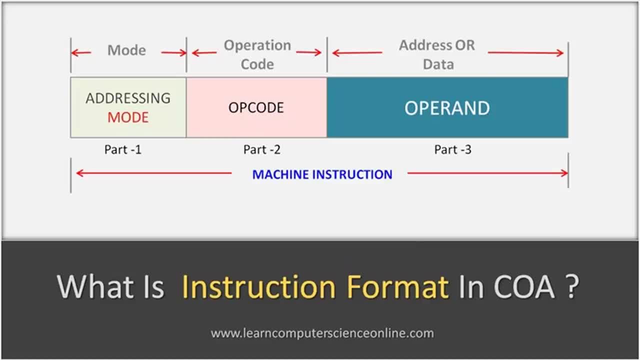 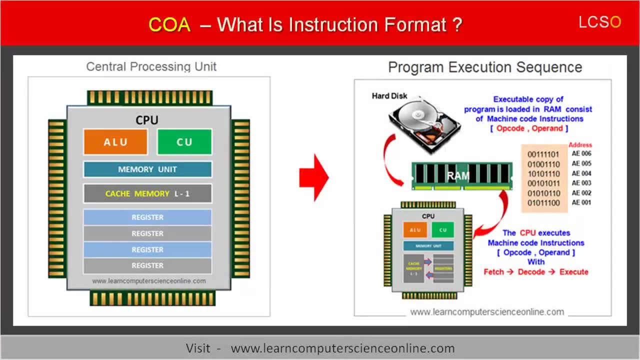 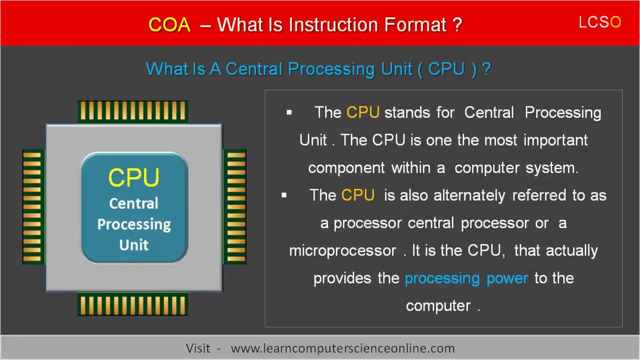 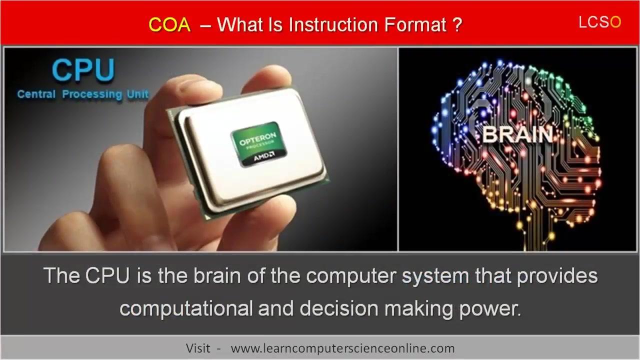 move on to another important concept in computer architecture, and the next concept is: what is instruction format? the concept of instruction format is related to how computer processor cpu decodes and executes the program machine instructions. the cpu stands for central processing unit. the cpu is the brain of the computer system, which provides the processing. 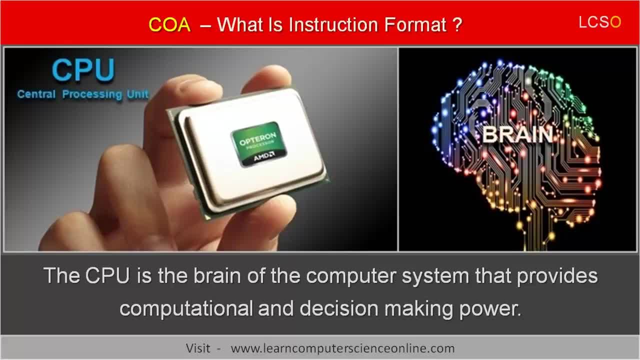 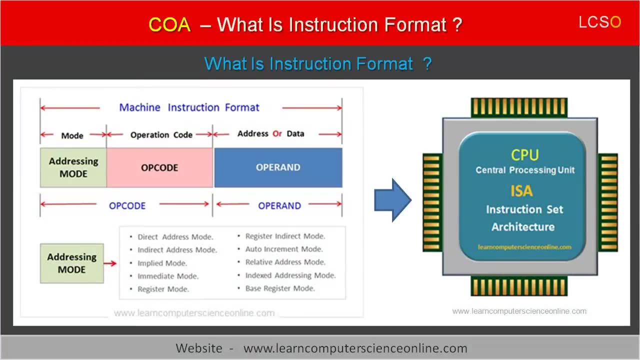 power to the computer system. the cpu controls all the operations performed by the computer system, including the activities necessary to execution the program. the cpu decodes and executes the program machine instructions based on the instruction format. at this stage the concept of instruction set architecture of the cpu also comes into picture. 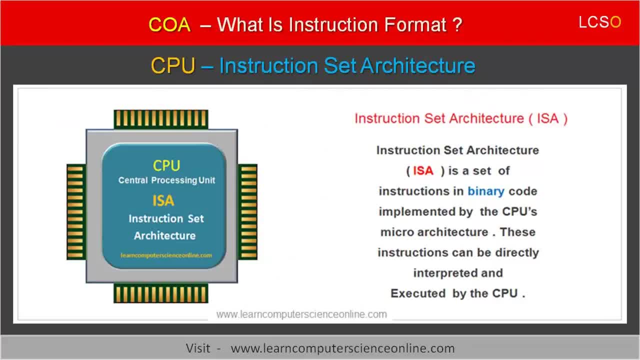 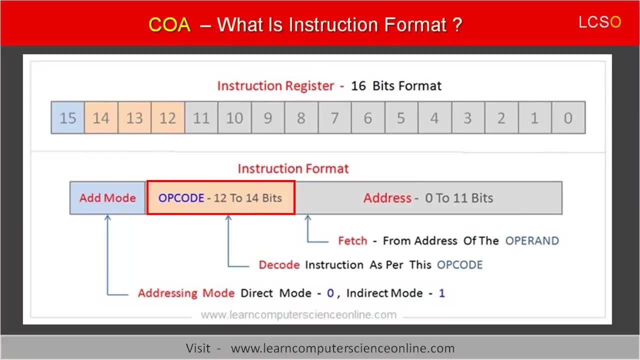 each microprocessor architecture implements a specific instruction set architecture and therefore the processor can support only machine instructions that can be mapped to its instruction set architecture commands. in simple words, the instruction format helps the cpu to find out the which operation to be performed, where is the data located and how to reach to the data. 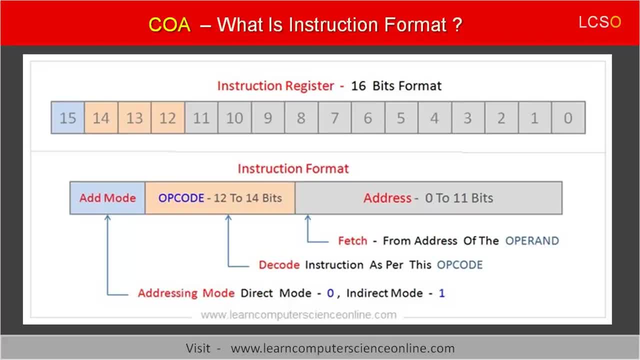 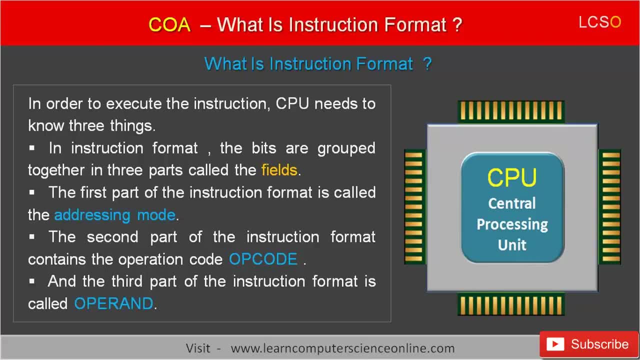 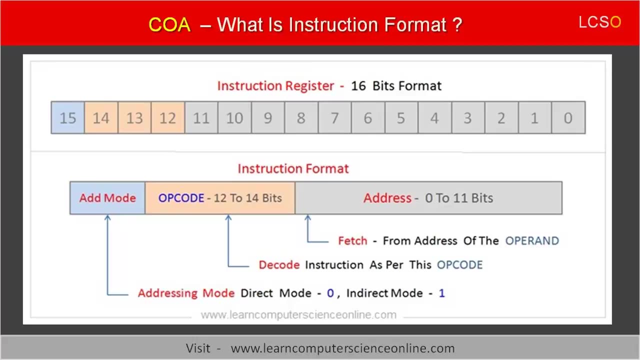 you can also use the cpu to perform the instruction set. architecture of the cpu. the instruction format provides all this information to the processor. in order to execute the instruction, cpu needs to know three things. in instruction format, the bits are grouped together in three parts called the fields. the first part of the instruction format is called the address mode. 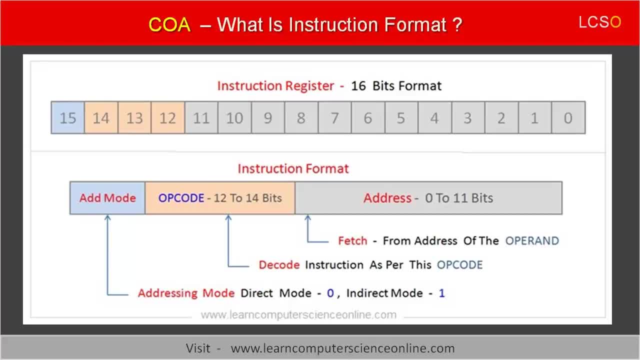 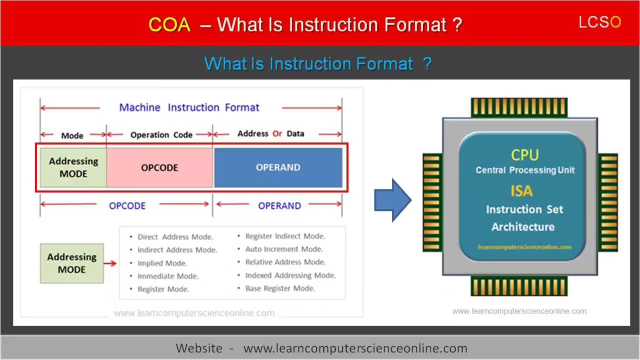 the second part of the instruction format contains the operation code, opcode, and the third part of the instruction format is called operand. the operand contains either the data or the operation or the memory address of the data. let us now study each of the three fields of instruction format in detail. 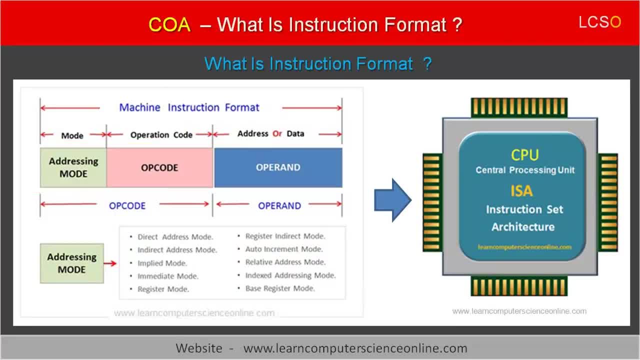 the first field of the instruction format as addressing mode. the data that has to be operated by the cpu can either be stored in the main memory ram, or it can be located in the cpu register. the addressing mode is the third field in the instruction format, represented by the sixteenth. 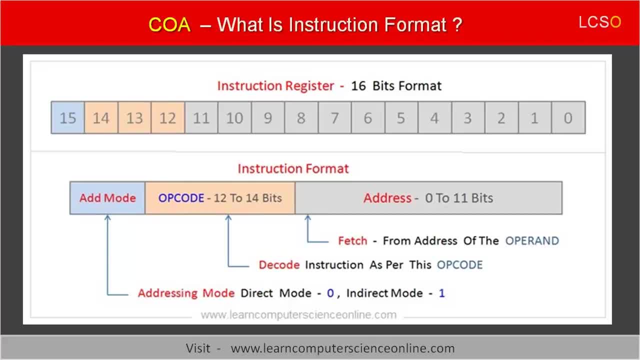 number single bit, for example. in sixteen bit instruction format the addressing mode is: The addressing mode directs the CPU to locate the data operand as specified in the machine instruction format. The next field of the instruction format is opcode. The opcode stands for operation code. 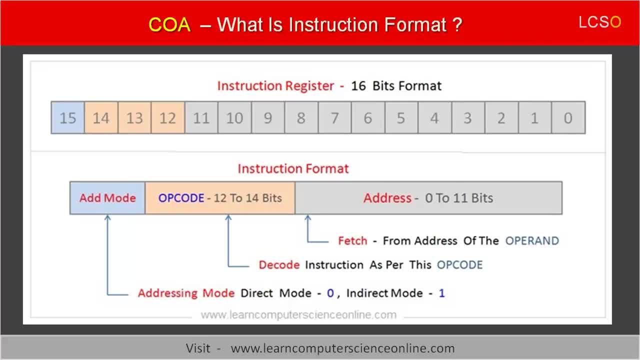 During the program execution the instruction is fetched into the instruction register, The instruction register, IR. The instruction register is a 16-bit register And a part of the IR is used to store the operation code For 16-bit instruction format. the group of 3 bits with number 12,, 13,, 14 indicates the operation code. 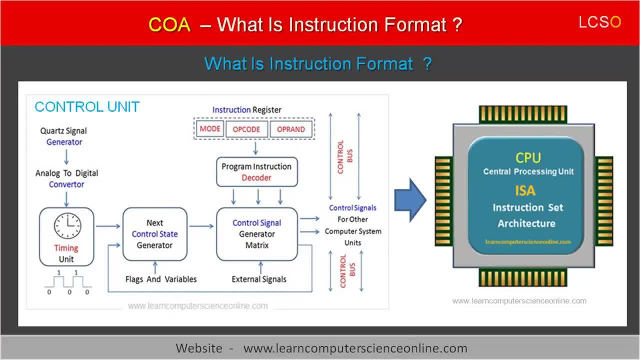 The operation code, opcode, is decoded by the decoder of the control unit. The control unit is one of the three important component of the microprocessor architecture. The control unit decodes the opcode as per the instruction set architecture of the CPU. The control unit generates the control signals for the ALU to execute the desired operation on the data.